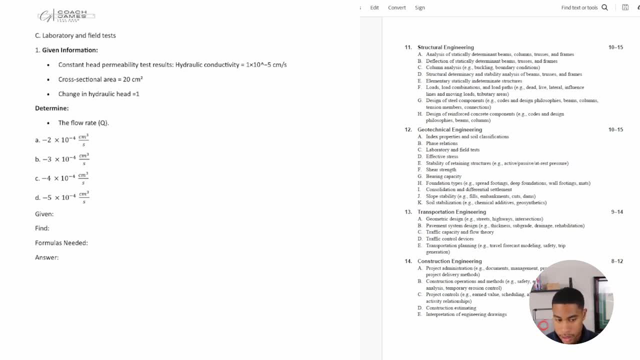 and then the information that I'm trying to find and any formulas that I may need to use, information that I'm given. I'm giving the hydraulic conductivity question, so we're just going do the forward control. So let's start it out, stick to. 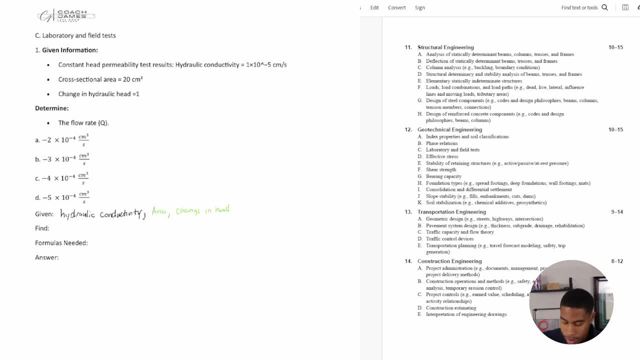 � are the float, we're in the head part here, we're asking the flow rate, or Q. trying to find the flow rate, or if I'm trying to find q, just from my knowledge of some of the practice that did in fluid 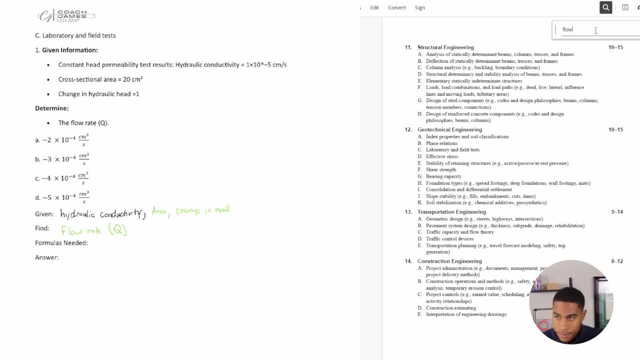 mechanics. I know that if I first, if I search flow, I get 278 results, So I'm going to try to use something they gave me to see if I can narrow down my formulas that I will can choose from. I'm going to search hydraulic conductivity, okay. 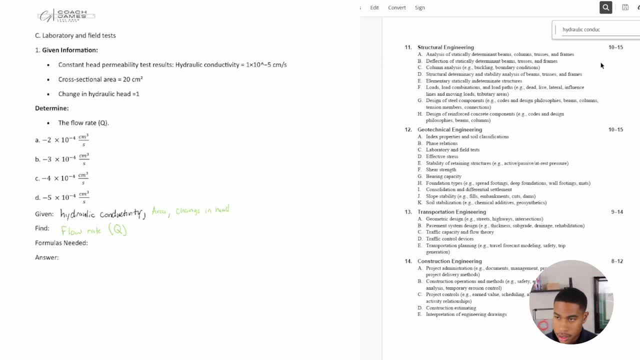 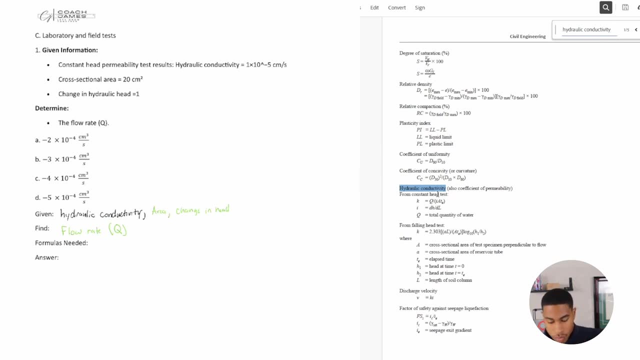 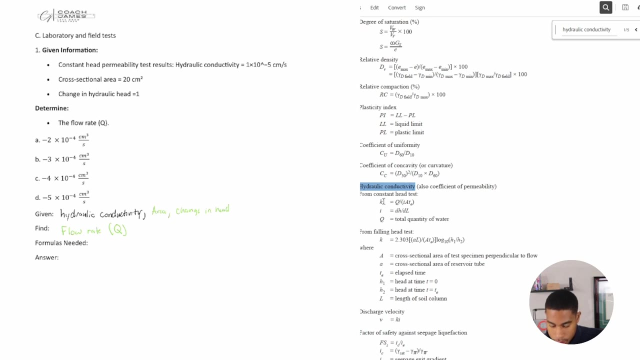 and only five results come up for hydraulic conductivity. I'm going to see if that's a variable that I can use to plug. Alright. so hydraulic conductivity here is going to be k, which equals q. q is the total quantity of water. Don't know what units those are, I, it's going to be change in. 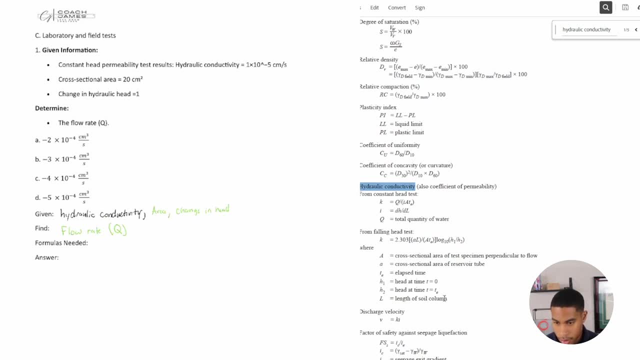 head over change in length. we are not given the length of the soil. column A: A is the cross sectional area test specimen. perpendicular to flow, Not necessarily, and this is a reservoir, And this is that there's a period of time that you need, So 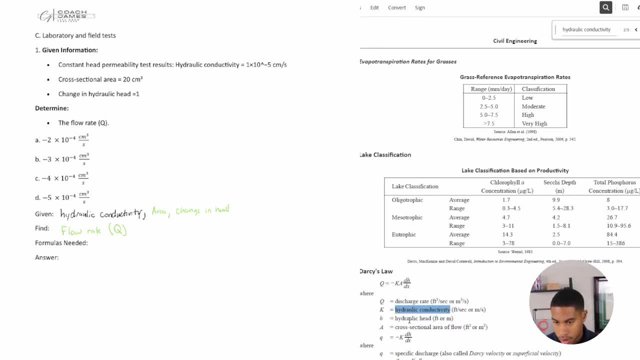 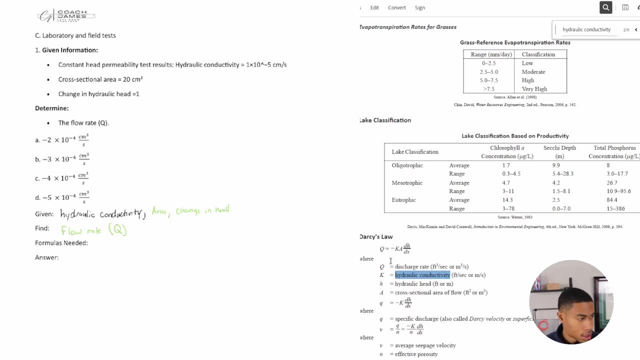 don't think that's the right formula, This one Darcy's law. we have a negative k, which is the hydraulic conductivity which we do have. What about a cross sectional area of flow? we have that, And then, so q is equal to negative k, So q is my flow. that 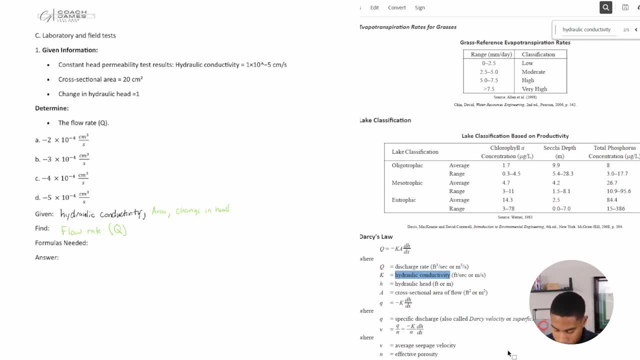 I'm searching for discharge rate, flow rate- same same thing. And then d, h over dx was d was h. hydraulic head. So it's the head, is the change in hydraulic head right? And so that would be one in this case. So I have all the things. 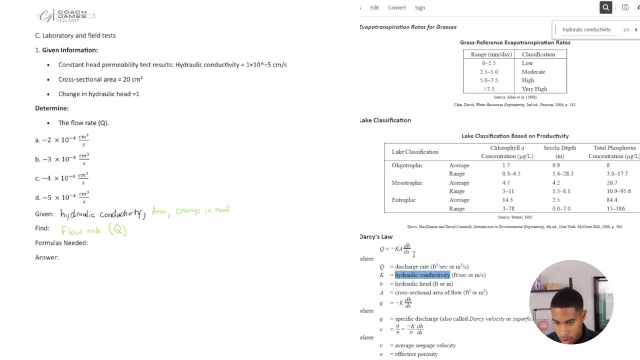 that I need in order to get my answer Alright. so let's write the equation out and then solve. Alright. so the form formulas needed is: q is equal to negative k, a and then d. eight over q is equal to negative h over dx. I'm gonna write out each variable: q is. 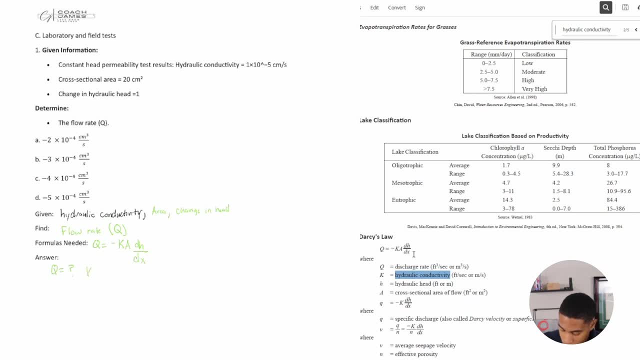 equal to question mark. So we're solving for k is equal to my hydraulic conductivity, which is one times 10, to the negative five centimeters over seconds. Key to know all of our my answer is in centimeters cubed over seconds. So if things are in, 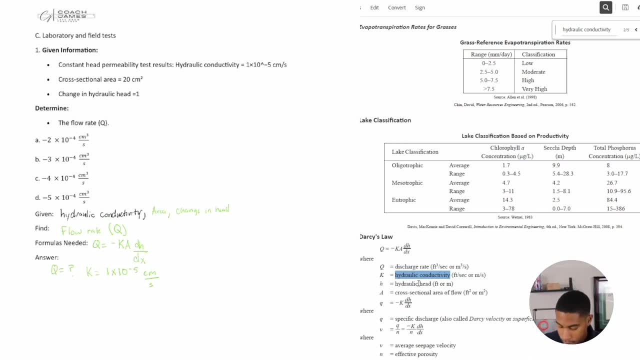 centimeters, or if things are in seconds, and that's perfect, Alright. a is equal to cross sectional area, which is equal to 20 centimeters squared, and then d, h over dx, equal to hydraulic head, or a change in hydraulic head, which is equal to one. Alright, so plug and chug q. 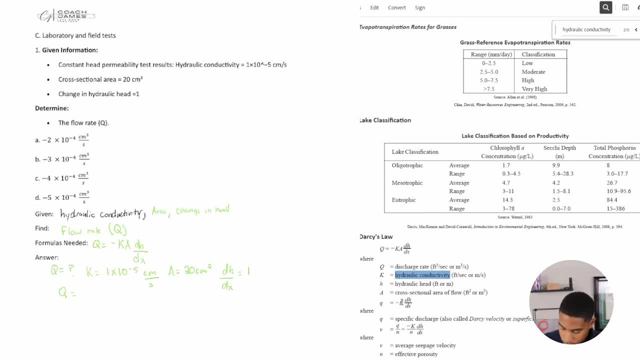 is equal to one or a negative k. negative one times 10, to the negative five centimeters per second. times my area, 20 centimeters square times my change in hydraulic head, which is equal to one. When I multiply all this out, I get negative two times 10. to the negative four centimeters. 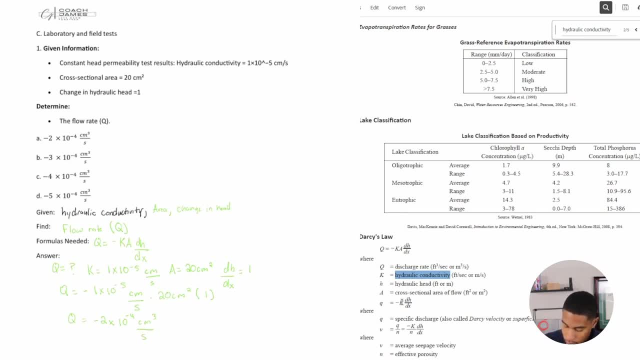 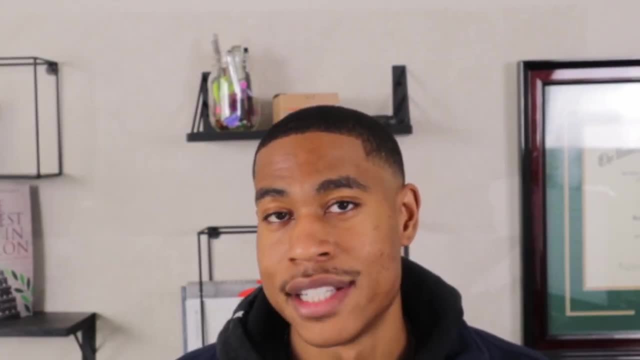 cubed divided by this Or same thing as a. Hey everybody. I know I didn't take time to formally introduce myself at the beginning, So I did want to let you know who I am and how I can best serve you as you're studying for your civil FE exam. So my name is James Huntley. 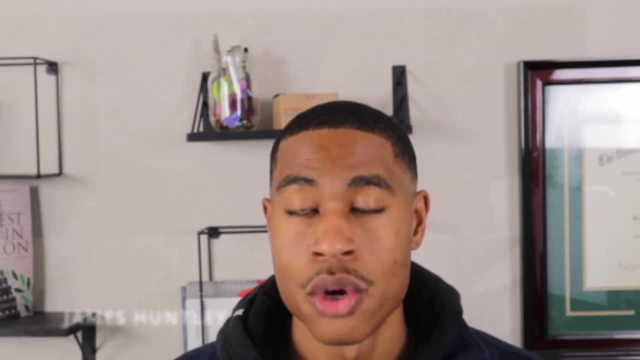 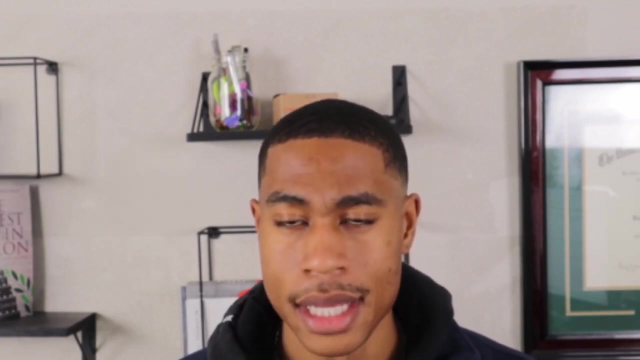 and I am a civil engineer who has helped hundreds of individuals pass and dominate their civil FE exam. Now I know this test is tough And as you're going through material, you may be saying I don't remember learning this stuff, Or 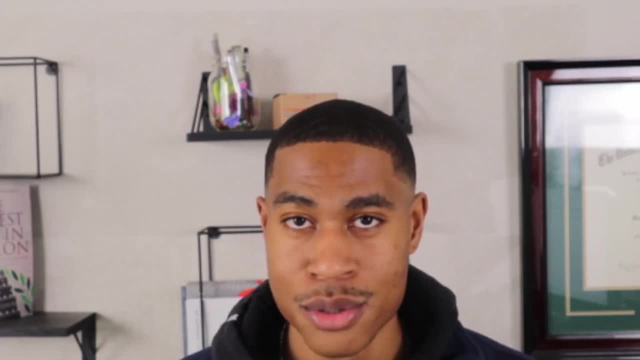 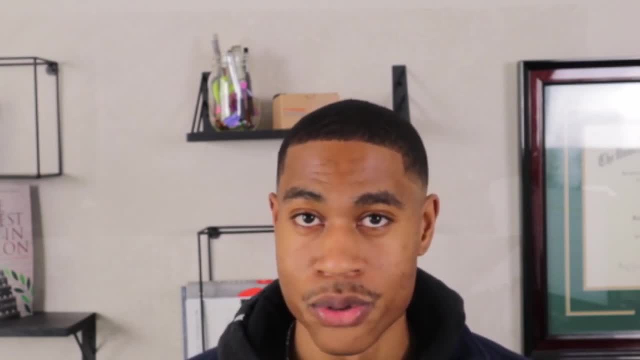 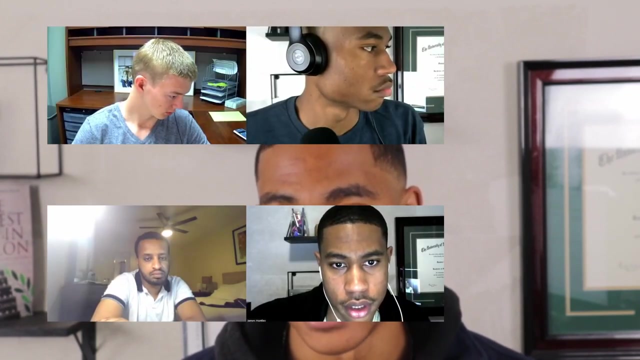 And there's so much material that you need to go through that it's a bit overwhelming. So I did want to let you know that I do help and work with individuals one on one to ensure that they pass their civil FE exam, And I've had individuals that have worked with me for 10 weeks. 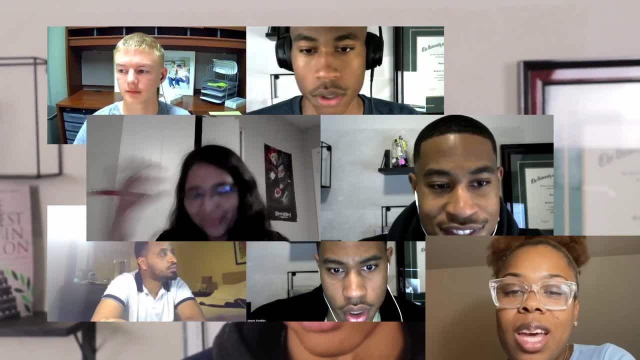 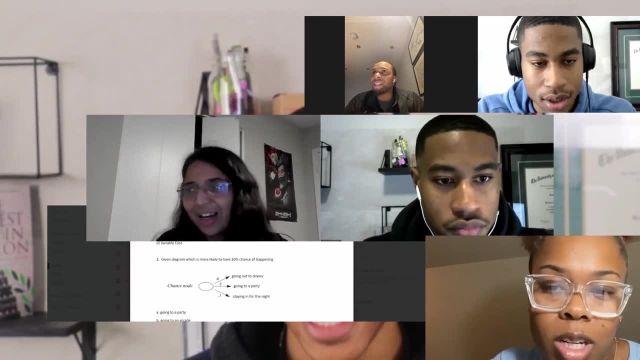 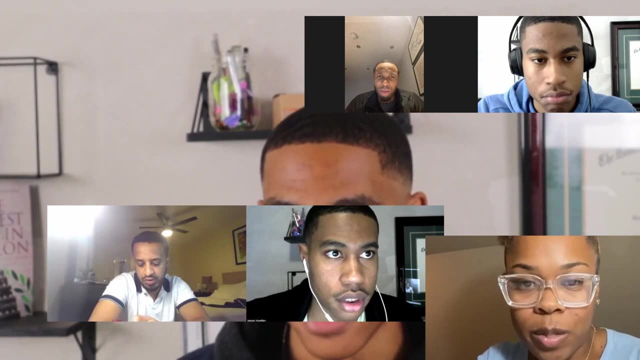 and that's the longest that has been, And I've had individuals that have worked with me for two weeks And we went back to back day after day after day, hours on hours on hours, putting in the work, working together to ensure that they went ahead and passed. And this exam is so important. 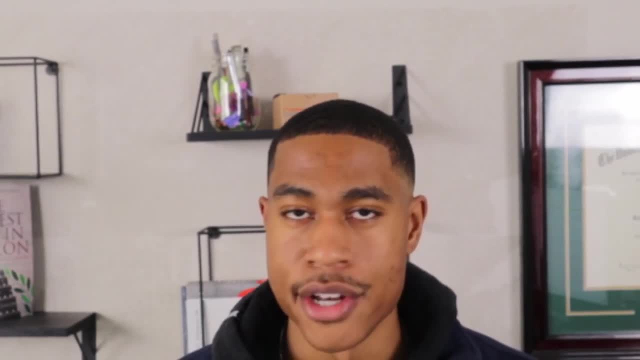 because I know that you want to make more money. I know that you want to, you know, get some promotions and be able to further your career and have your PE. So definitely want to open and extend a hand out, Want to be able to save you time, Right, Because I know some people that watch. 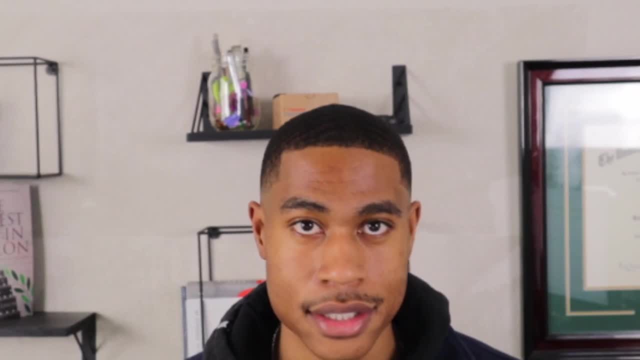 my videos. you may have been watching my videos for six, nine, even 12 months and you still haven't passed your civil FE exam, And that is the one thing that's keeping you from making more income or impact And furthering your career. So it's definitely costing you money, resources, everything. So 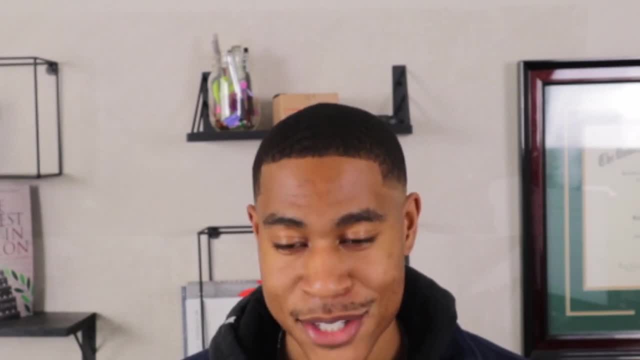 looking to create more success stories. I am looking to work with individuals one on one. I want to hop on Zoom with you. I want you to share what you're doing as you're solving these problems, so I can spot out what you may be struggling with and open your eyes so that. 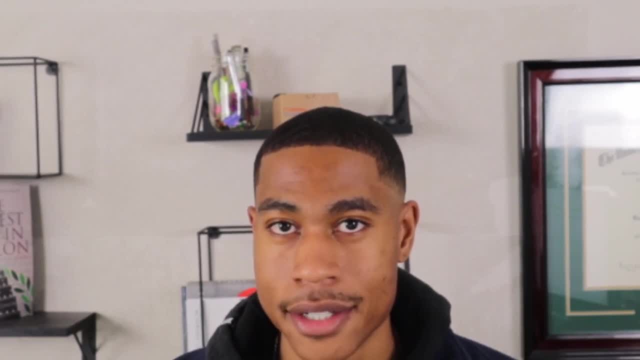 you're not going into This test completely blind. Now, for some of you, you may have failed a test once, twice, had some people fail five times, or you may be wanting to take this test initially and you just want to make sure that you pass it up front. So do you have one on one services? 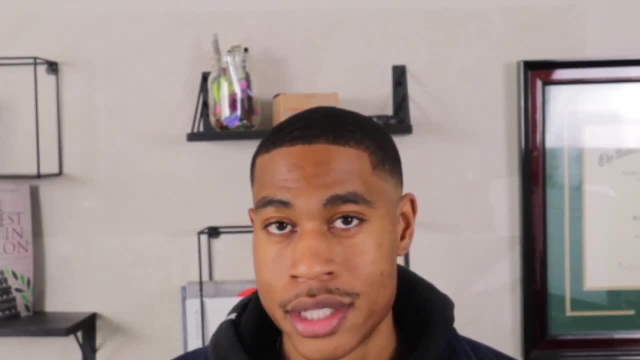 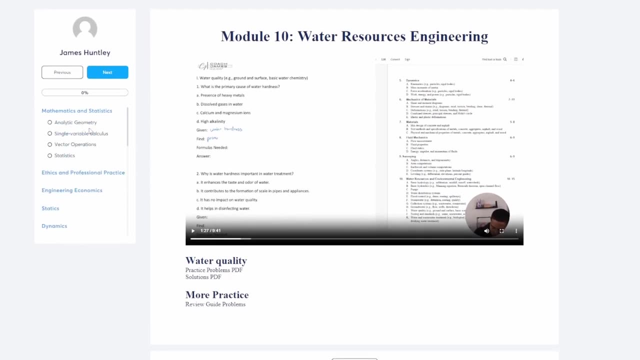 I also have some do it yourself courses that if you're like: no, I got this, I got it all on my own. I know everything, Or I'm I'm going to take the time to study everything- I do have some resources and materials to be able to help you in that way. 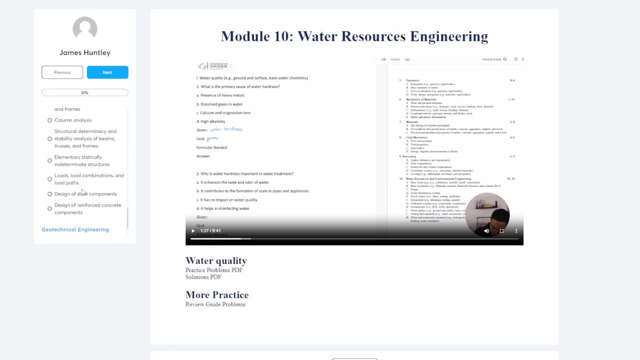 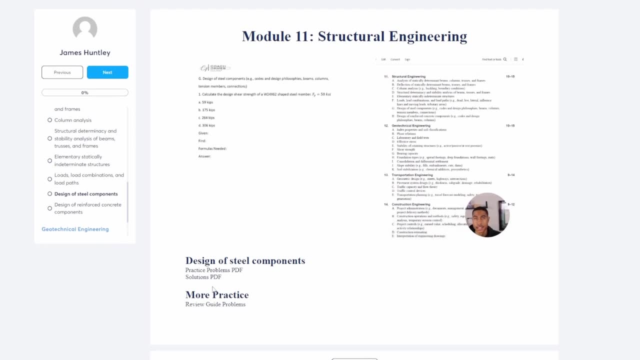 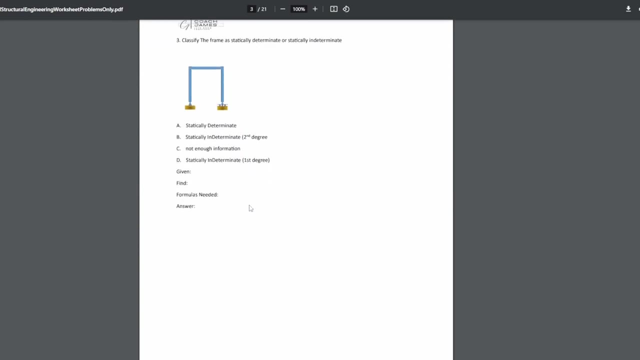 But my biggest fear is that you're investing in something- these programs or these courses- and you know you're not getting back or having proper feedback to help you and to push you forward. You're just given a bunch of information and no one's sharing with you what you may be actually. 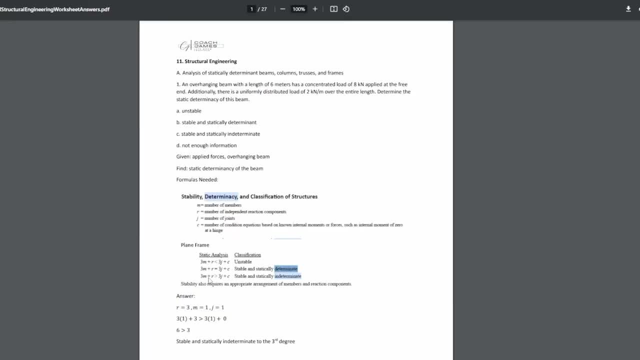 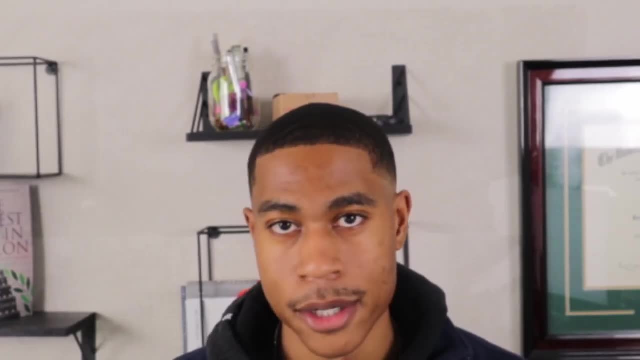 struggling With or what's keeping you from passing your F exam. So looking to create a ton of success stories? so feel free. down in the description box below. I have a ton of resources, including one on one coaching. top on a call.